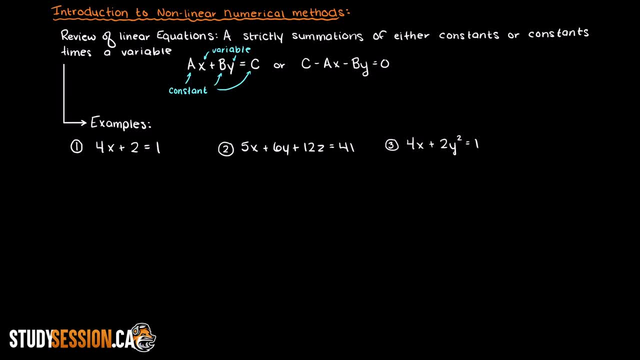 Alright, so this first one here is just a summation of variables times constants and is therefore a linear equation. Additionally for this second equation, there are only summations of variables times constants. However, for equation 3, here we do have a summation of variables times constants, or just variables. 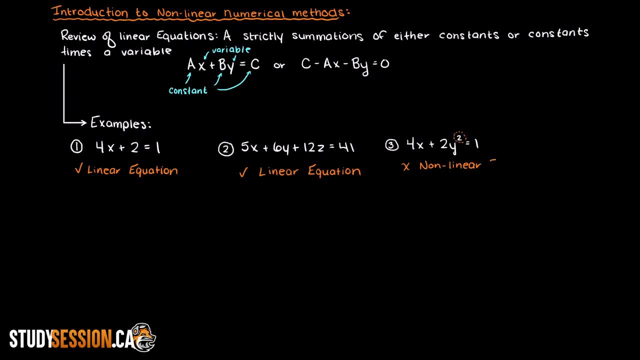 However, the last term is a squared variable and this makes this equation non-linear. Any terms that violate our constant times, a variable or just a variable rule, makes our equation non-linear. So what exactly does this mean to solve a non-linear system of equations? 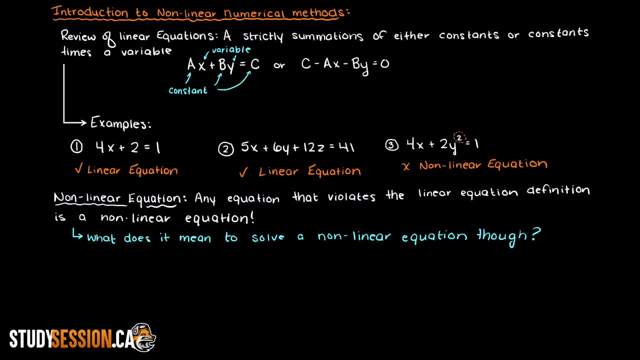 or just a non-linear equation. Well, to solve a system of non-linear equations means to find the roots of the function, That is, to find where the function crosses our x-axis. So, graphically, if we had a graph that looks like this: 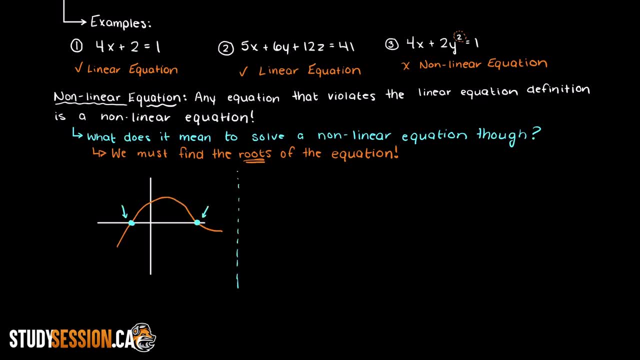 we would try to identify these points here on our graph. You are already familiar with one of these and that is the quadratic formula which solves for the roots of a parabola which is mathematically non-linear And graphically can look a bunch of different ways, but here are a few. 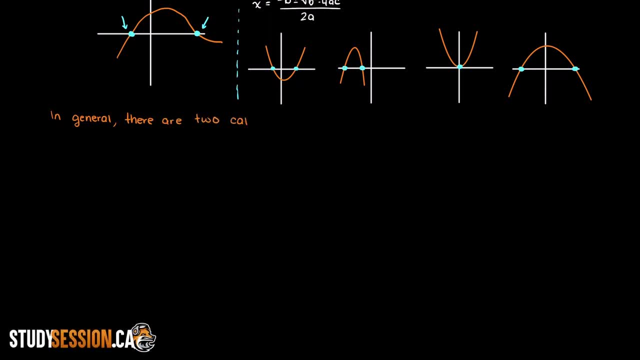 In general in non-linear numerical methods, there are two categories for solving for the roots of functions, and these are known as closed or open methods. We will go more into detail about these two methods in future videos when we talk about more specific ideas, formulas and methods used. 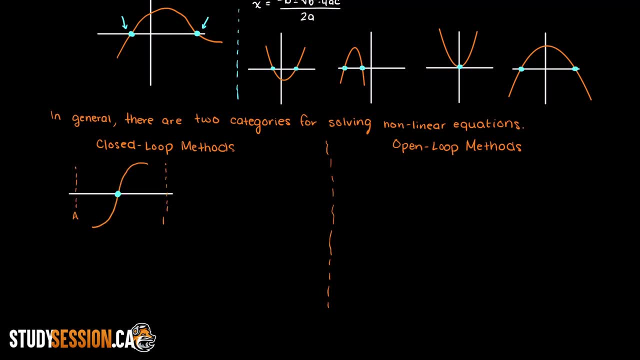 However, in general, closed methods are used when a root is known to be within a specific range. However, if you do not know that there is a root within a specific range you specified, or if there is more than one root in the section, then you will not get an answer, or at least 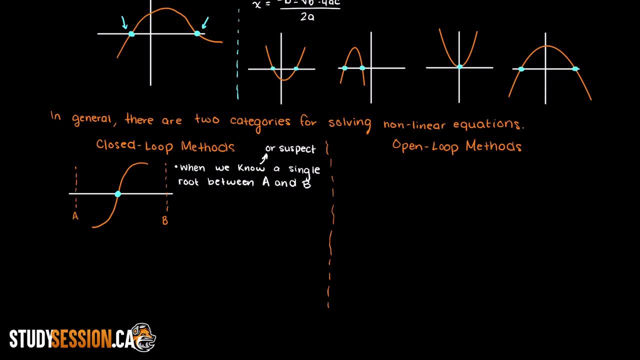 not one that makes any sense. The other method is called an open method. Unlike the closed method, the user does not need to define a range. rather, they state an initial starting point. This is an initial guess where they think the root might be, and this is used in various 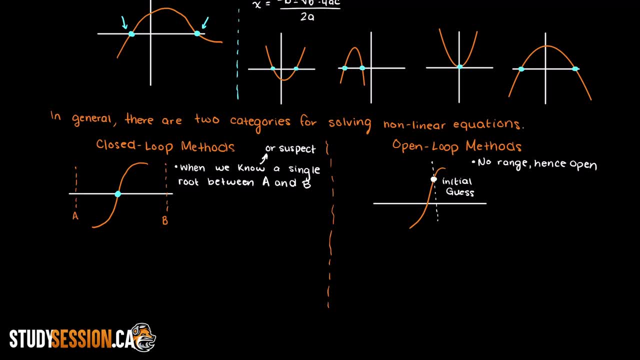 algorithms to estimate where the root of a function will be. Sometimes this does not work, though. however, choosing a proper starting point will more often than not solve this issue. We will talk more about resolving and confronting these issues more in future videos, though.